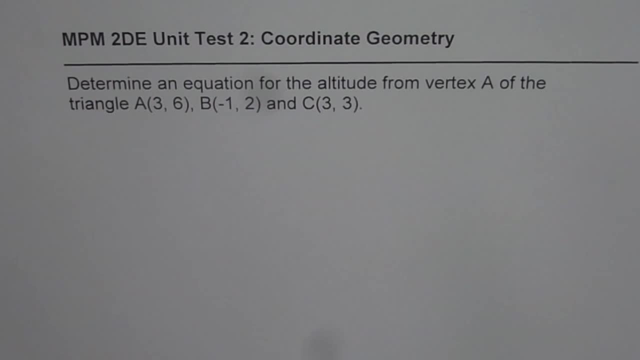 avoid these as ultimately they count a lot. The question here is: determine an equation for the altitude from vertex A of the triangle: A- 3,6,, B is minus 1,2 and C is 3,3.. This is a good idea to first sketch. Now, whenever we are trying to sketch a triangle like this, 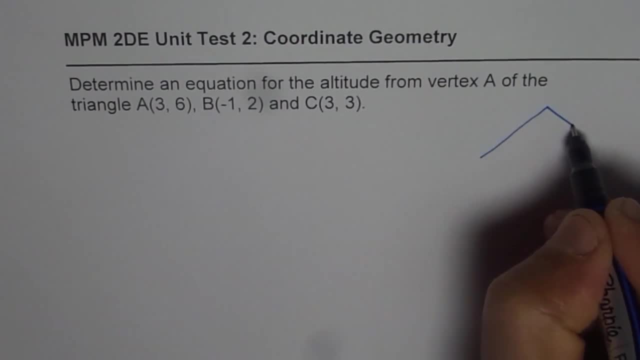 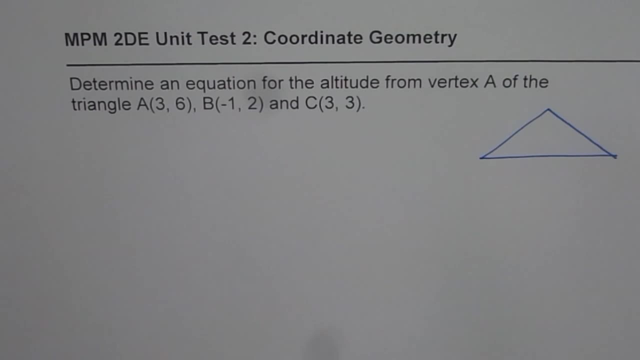 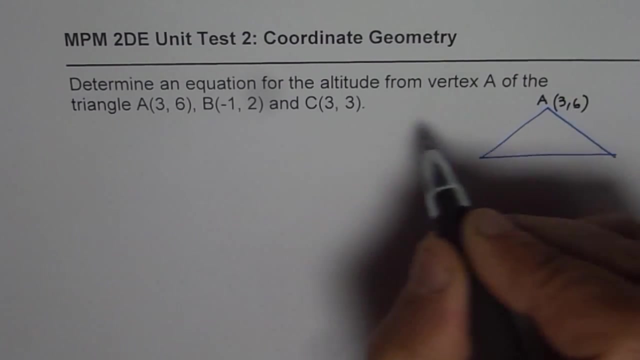 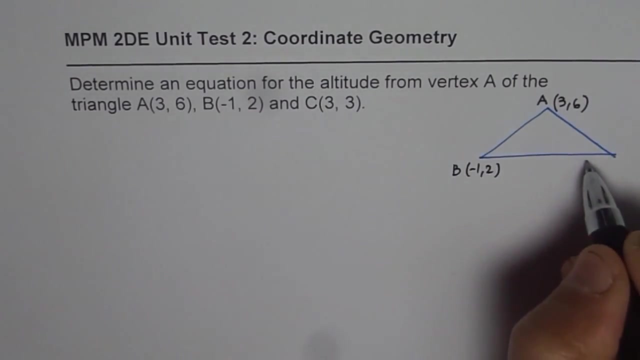 we need not really make a coordinate system and then sketch it. We can just make one approximate sketch convenient to solve the problem. So let us say this is our sketch for the triangle. Here is the vertex: A is 3,6, B is minus 1 and 2 and C is 3,3.. So that becomes the three vertices. 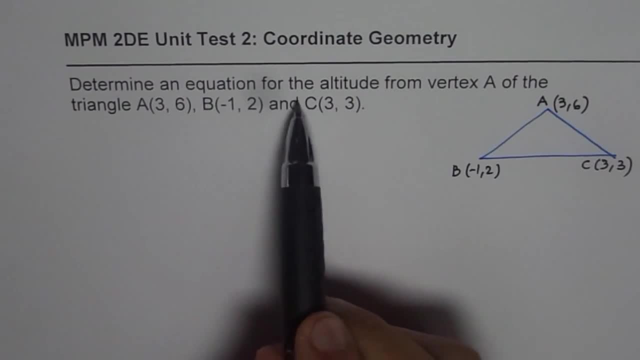 of the triangle, We need to find equation of the altitude from the vertex A. Now, altitude really means that you have to drop a perpendicular from the vertex. So if you drop a perpendicular from the vertex, it would be at right angles to the opposite side. So that means: let this. 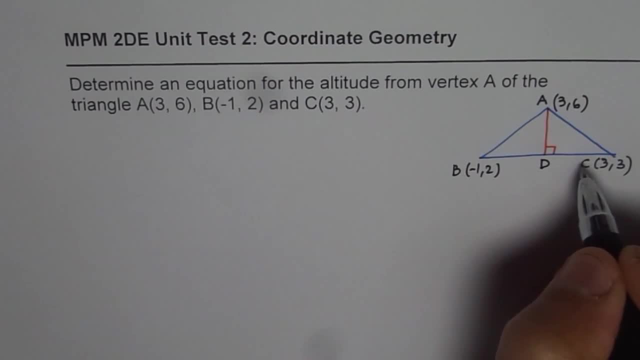 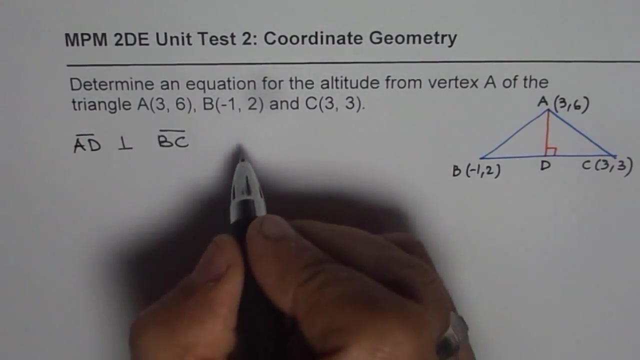 point be D, right. So AD is the altitude for us. Now. AD is also perpendicular to the side BC, right. since we have dropped a perpendicular, That really means that slope of AD- let me write, slope of AD- is a perpendicular slope to the opposite side of the vertex. So if we have 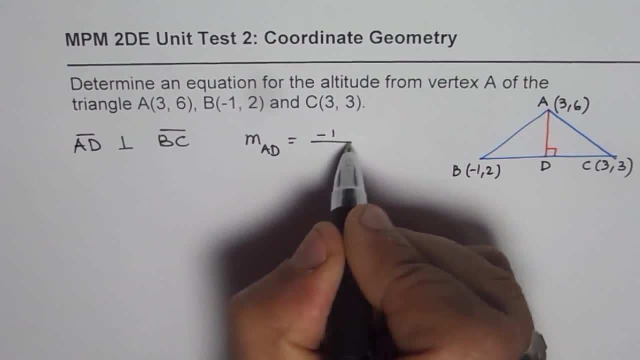 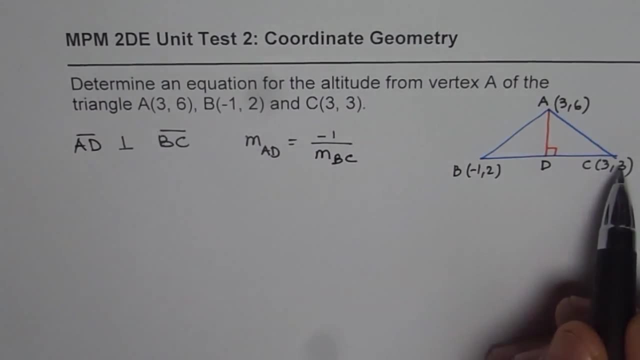 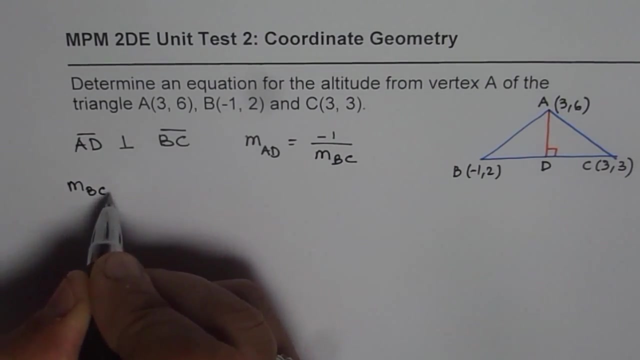 should be equals to negative reciprocal slope of BC. so from the given points we can always find the slope of BC. so let's do that. so first step is find slope of the line segment BC, which in this case will be Y 2 minus Y 1 divided by X 2. 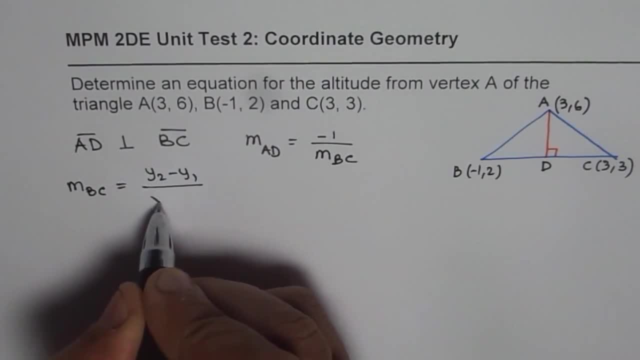 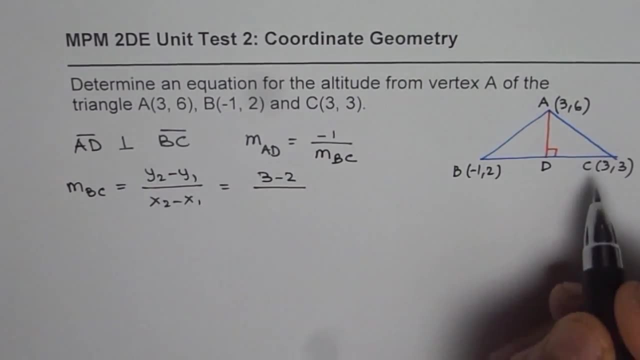 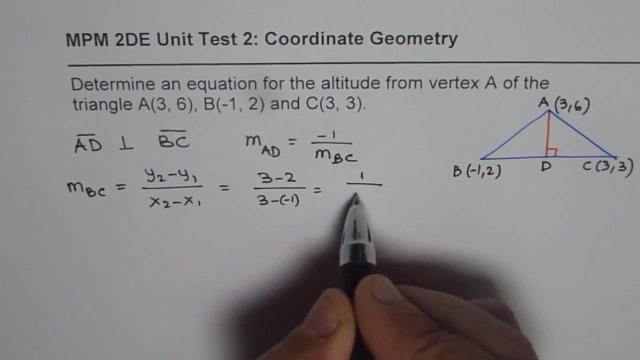 minus X, 1. that's the formula right now here: 3 minus 2 divided by 3 minus minus 1, so 3 minus minus 1, 3 minus 2 is 1 and that becomes 4. so that is the slope of BC. 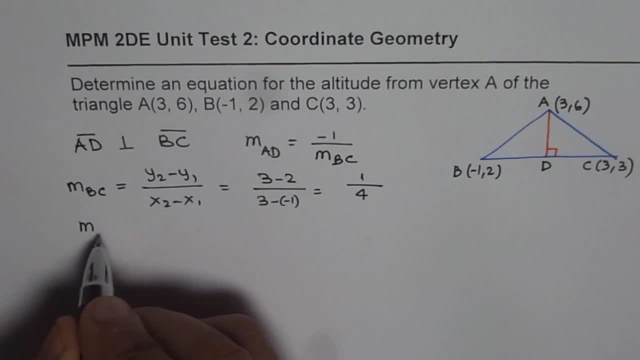 so what is the slope of perpendicular? so the altitude slope AD will be equal to negative reciprocal slope of BC. so what is the slope of perpendicular? so the altitude slope AD will be equal to negative reciprocal of this that means negative of. I should write 1 over 1 over 4 that. 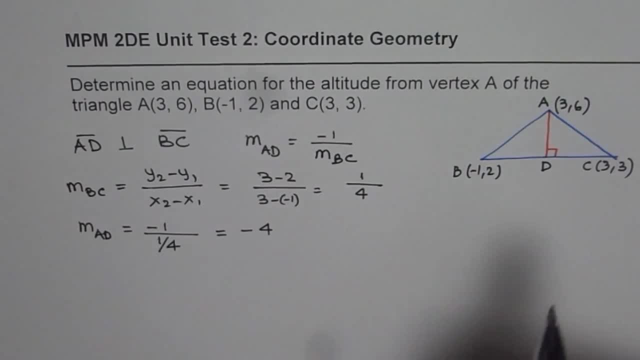 makes it negative 4, right? so the slope for us is negative 4 for AD. once we know the slope, we can find the equation using one of the points. so now equation of altitude should be: so we are considering the point a. let me write point a as 3, 6 and slope M of the. 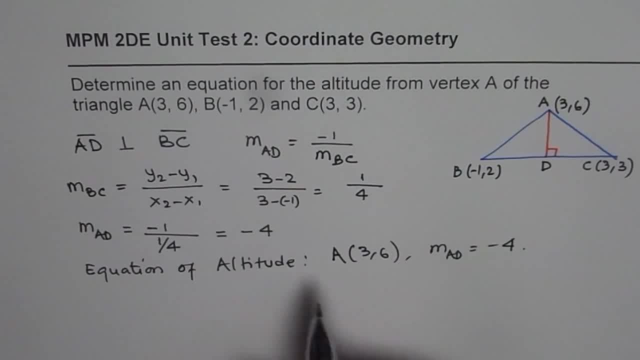 altitude AD is minus 4. we can write it like: y equals to MX plus P. could be this question of the line where we know slope is minus 4. so we'll write minus 4. for M. for X, we'll write X value of 3. 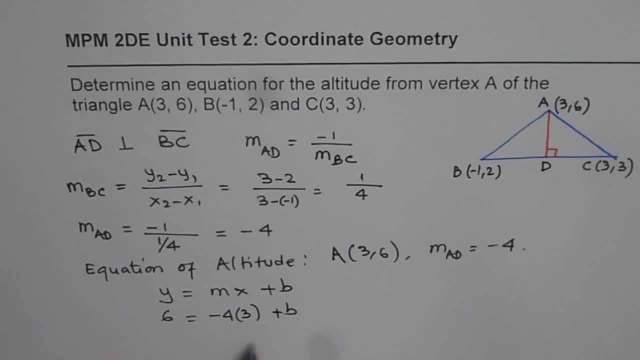 we need to find B, the y-intercept, and by value 6 so we can solve for B from here. 4 times 3 is 12, with minus 12. we can take it on this side. so add 12 on both the sides so we get 6 plus 12 equals to minus 12 plus B plus 12 and that gives. 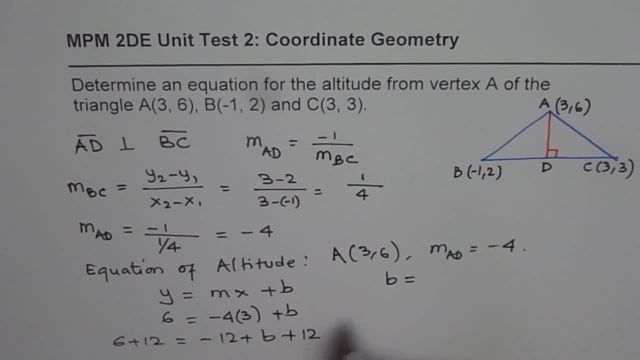 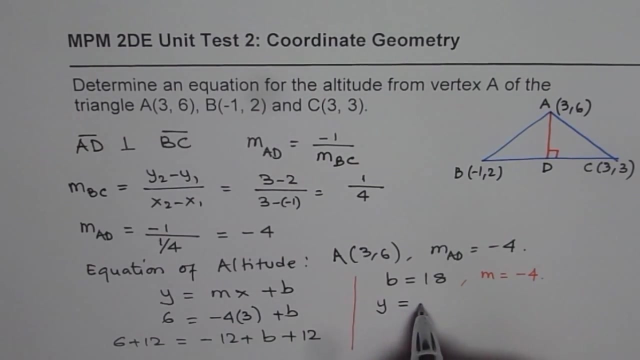 us the value for B, so we get B as equals to 18, right? so that is how we can find the y-intercept. now we already know slope is minus 4, right? so therefore the equation of the line is: y equals 2mx, which is minus 4x plus y. intercept of 18, right? so that? 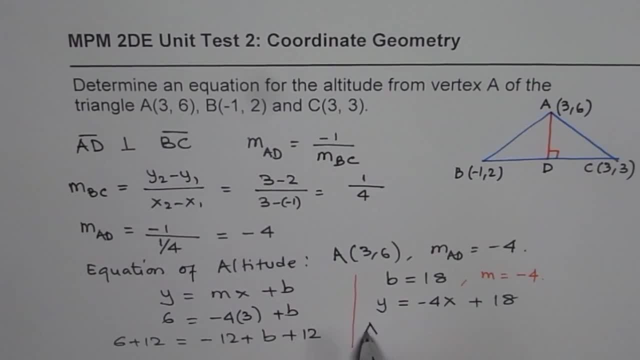 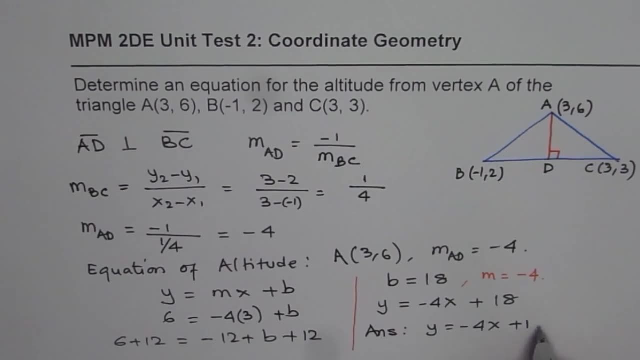 becomes the equation of the altitude, right? so that answer is: equation of the altitude. is y equals to minus 4x plus 18? it's kind of important to write down all the steps in a times. give reason to get full marks, otherwise you might just lose 0.5, 0.5 and they add up. 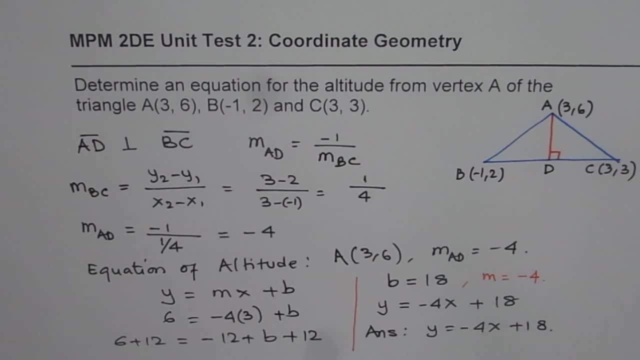 i hope that helps. thank you and all the best.